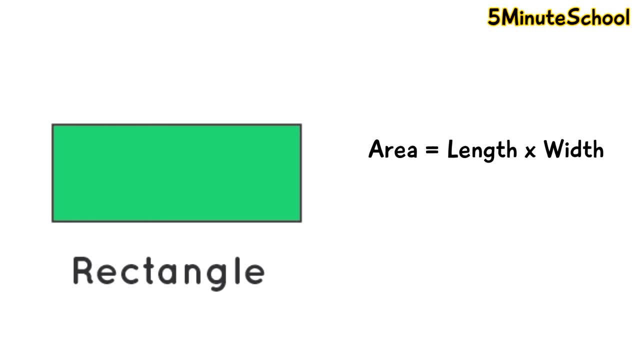 The length and width are going to be different On a rectangle, but all you have to do is times them together to get the area of the rectangle. For example, for this rectangle here, the length is 6 centimeters and 3 centimeters. We just times them. 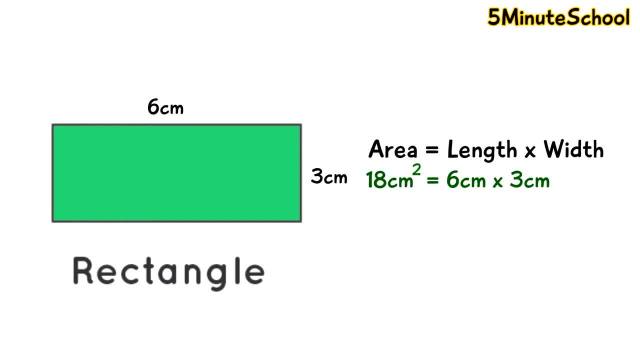 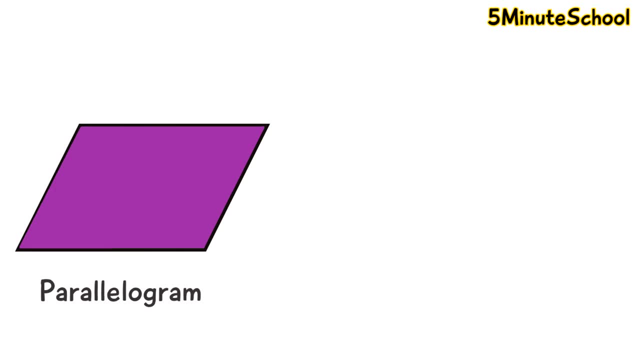 both together and we get the area, which is 18 centimeters squared. A parallelogram looks like this: It's a four-sided shape with two pairs of the sides at equal lengths. Essentially it's a rectangle, but two sides are angulated. You need to work out the area of a parallelogram in the same. 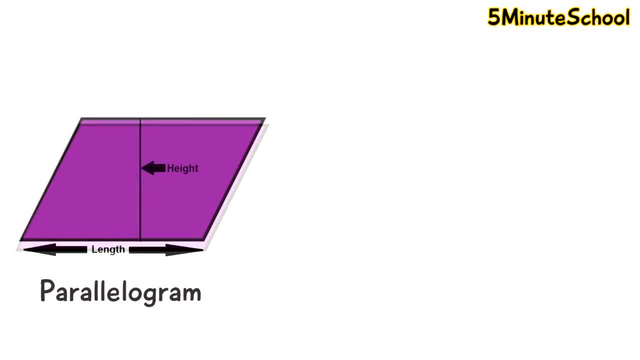 way you would work out the area of a rectangle. So you're going to need a square and a square. So you're going to need a square and a square. So you're going to need a square and a square Of a rectangle. you multiply the height by the length. You don't measure along these. 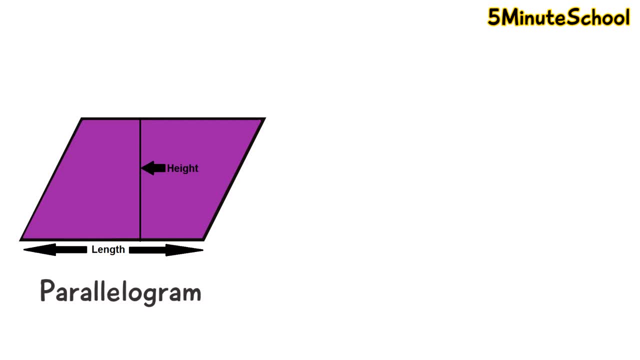 angulated sides, as it would distort your measurements. So essentially, the area of a parallelogram is the length times by the height, like so. So for this parallelogram here, we're going to times the height, which is 8 centimeters, by the length here, which is 6 centimeters. 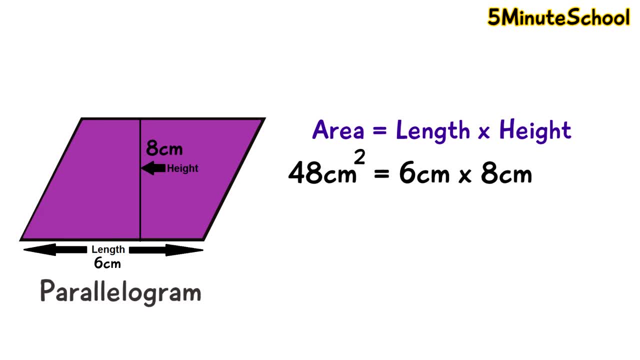 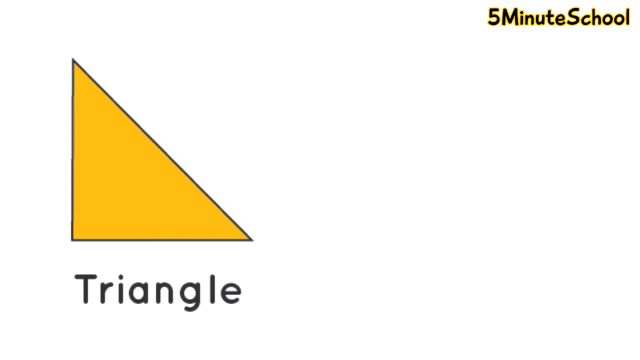 And then we can work out the area, which is 8 times 6 centimeters, which is 48 centimeters squared. To work out the area of a triangle, you have to remember that a triangle is basically half a square or half a parallelogram. Essentially, all you need to do is just find out the height and width. 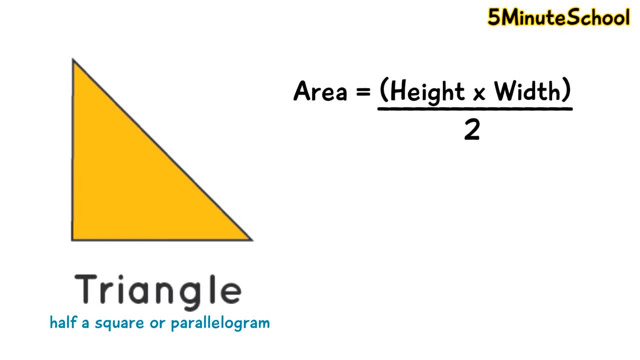 multiply them together and then divide it by 2.. So let's look at these two examples. The height of this triangle is 5 centimeters and its length is 4 centimeters. That means the area of the triangle is 5 times 4, which is 20, and then divide that by 2.. That gives you 10 centimeters squared. 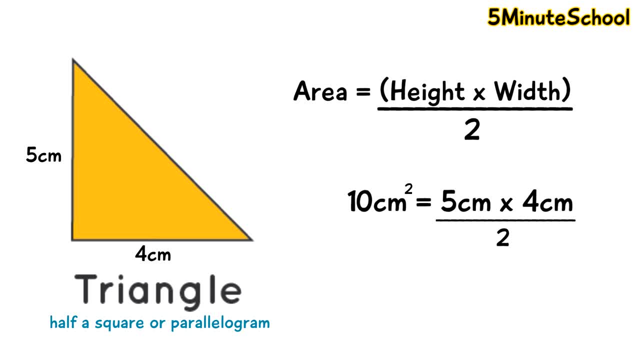 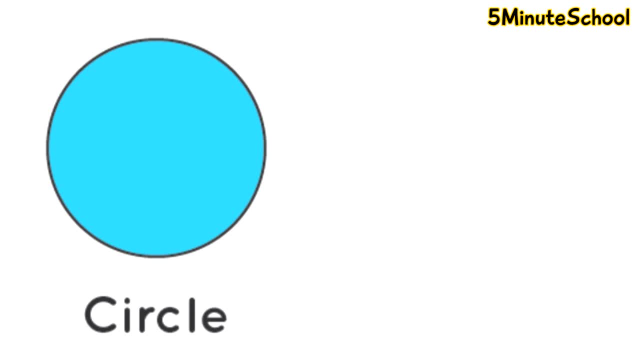 So that's how to work out the area of a triangle. Lastly, we're going to teach you how to work out the area of a circle. There are some things you need to know about circles before we start. So the length of a straight line from one side of the circle to the exact opposite side which passes through this? 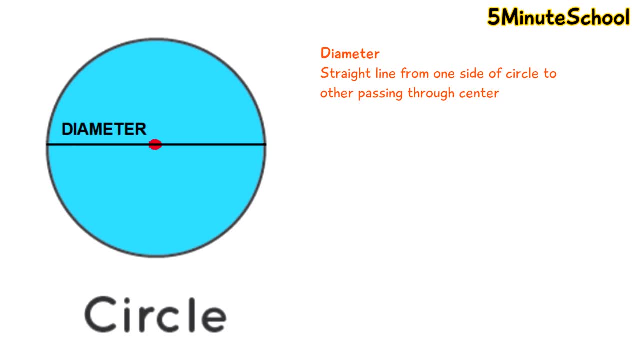 middle point here of the circle. This length is called the diameter. The radius of the circle is aligned. from this midpoint here of the circle to the edge, The radius is actually half the value of the diameter. So the radius of the circle is actually half the value of the diameter. So